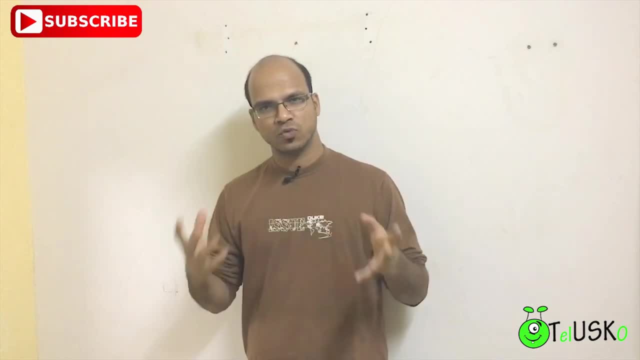 a ores in that. now, depend upon which, what type of ores you want to go for. maybe you want a open source ores, you will be going for android. if you want a closed source ores, you will be going for ios, and if you want some weird ores, you will be going for windows, right, so we have depend upon. 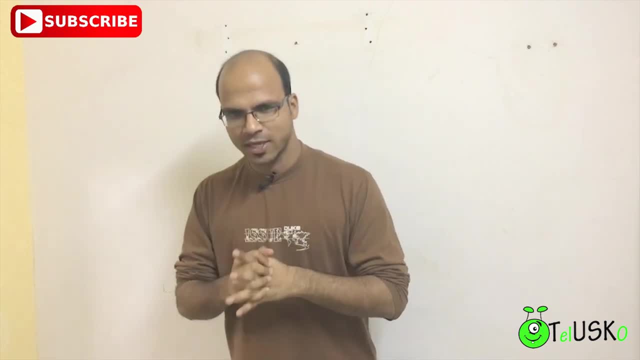 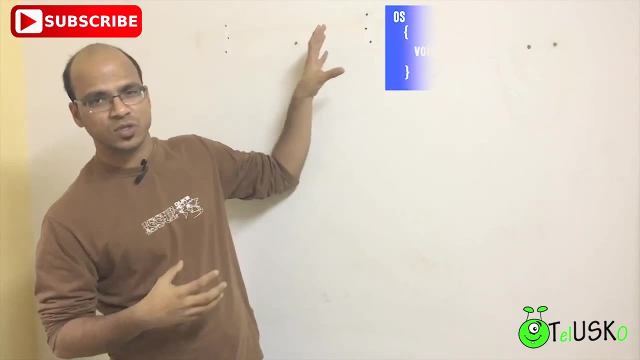 your requirement, you'll be having different, different types of ores, right? so let's say, you, you have a main method and in that main method, you want an object of ores now. so you'll be having an interface which is ores, and this ores interface will be implemented by android, ores, ios and 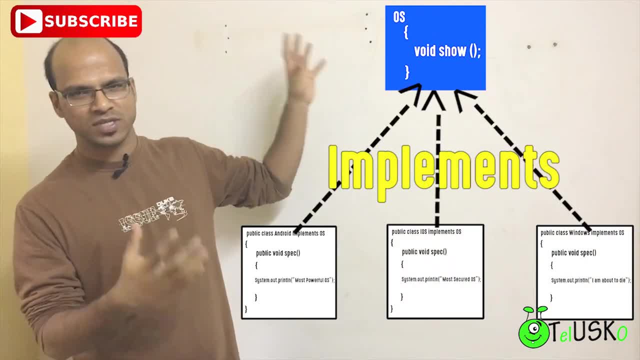 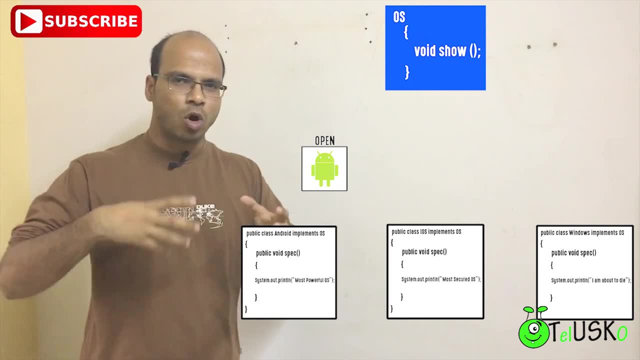 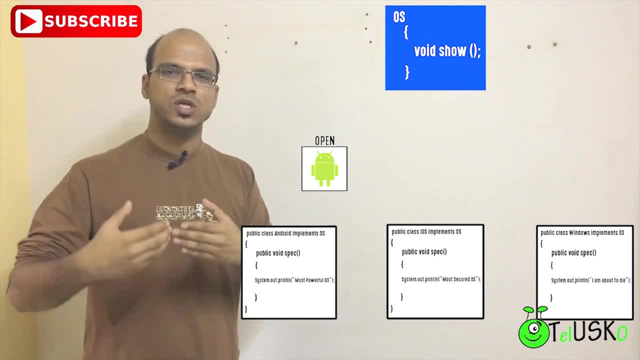 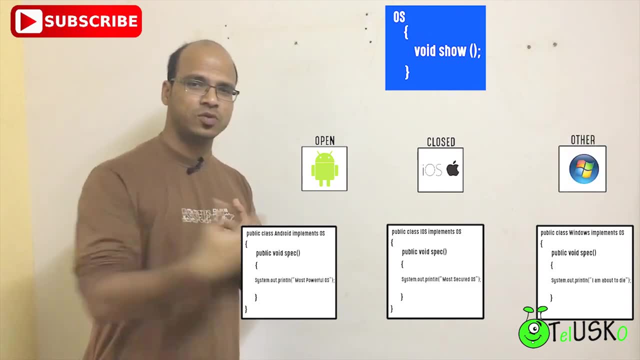 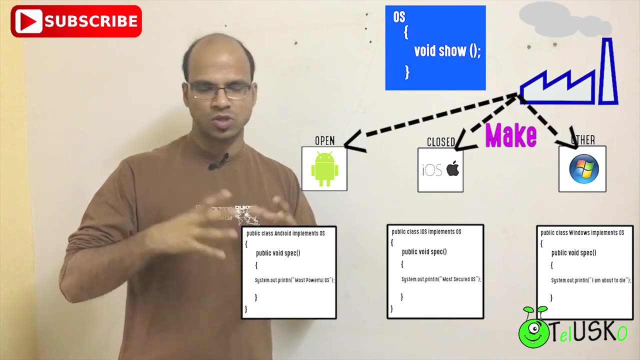 of android phone, android os. if you want a os which is closed source, you will get automatically. you will get object of ios, right? so somebody else is providing you that object and that somebody else is your factory. okay now, because when you talk about software development or software development, 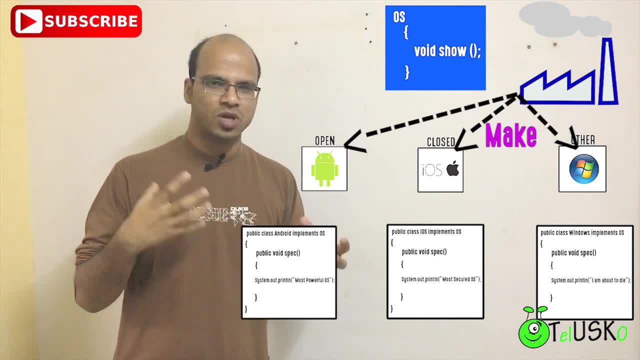 life cycle or software engineering, whenever you build a project, so you have to work with different modules, right, and all this module should have low coupling and high cohesion. so you, if you want to achieve this low coupling, we- we use something called as factory here. so instead of you creating 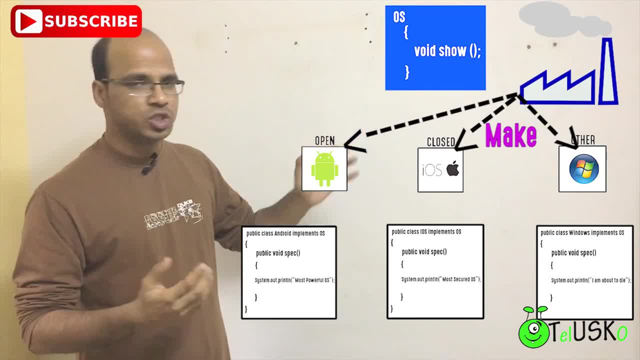 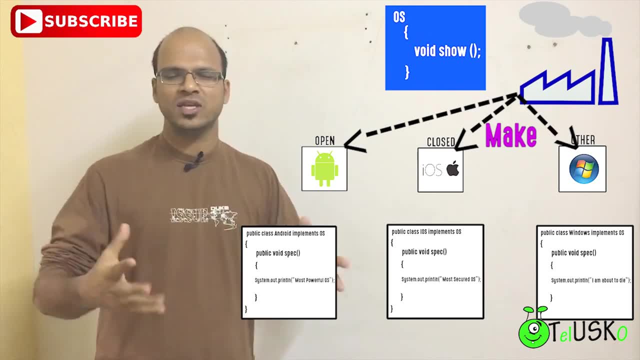 this object. ask someone else to create you this object. so maybe in future you'll be, you'll be having a new os. so let's say you have a os, maybe, i don't know, maybe symbian it's an old os. right, let's say you have symbian one more, so you have one more class there. so as a normal user you are. 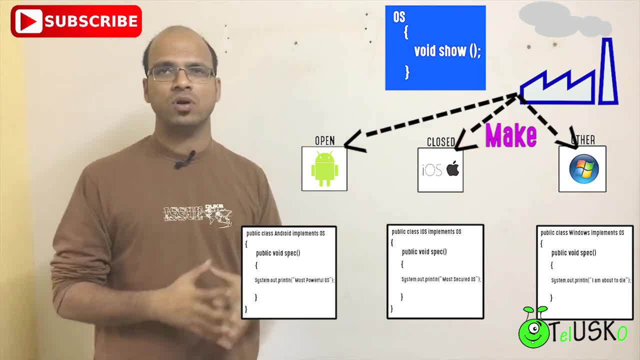 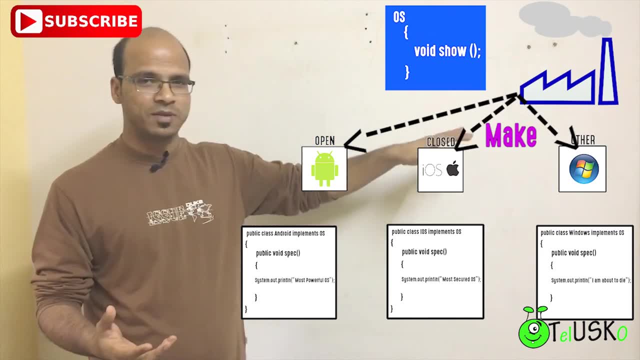 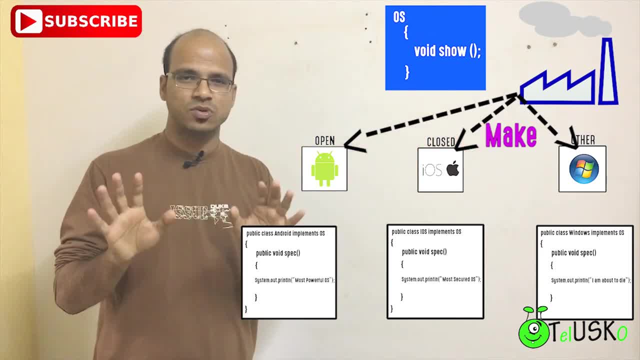 replaced by blackberry os. you don't know about anything, right you just. you just have to specify old os automatically you will get blackberry object. who is giving those objects? it is your factory. and how to implement all these things that we'll see in the practical session.